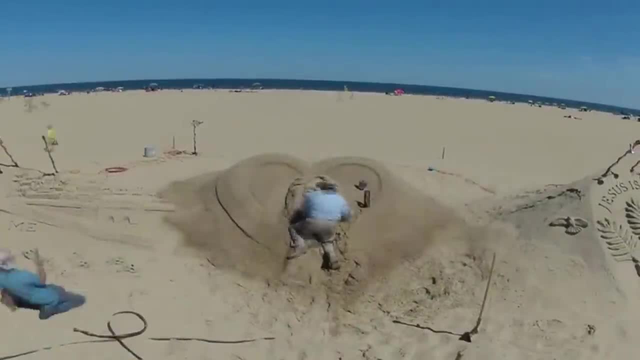 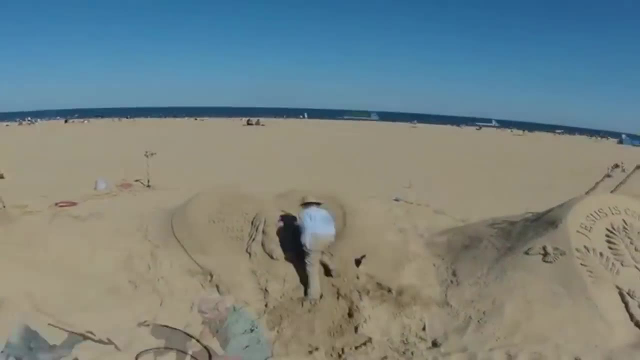 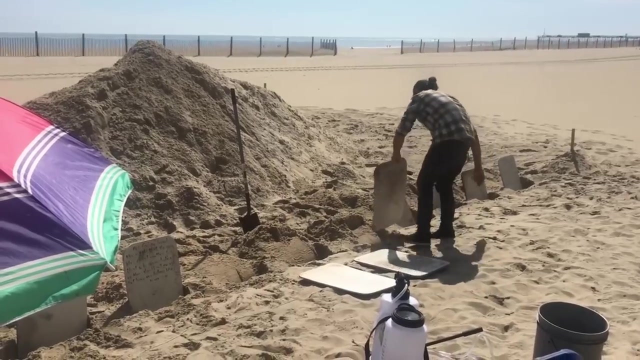 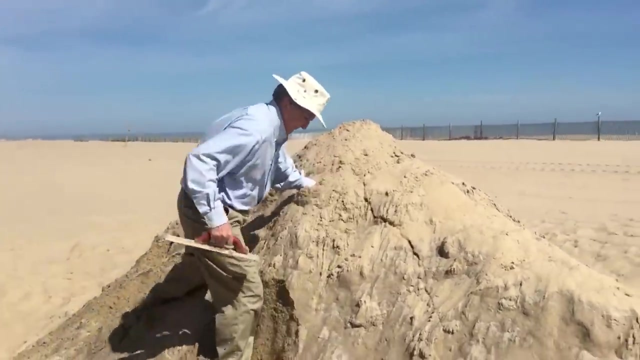 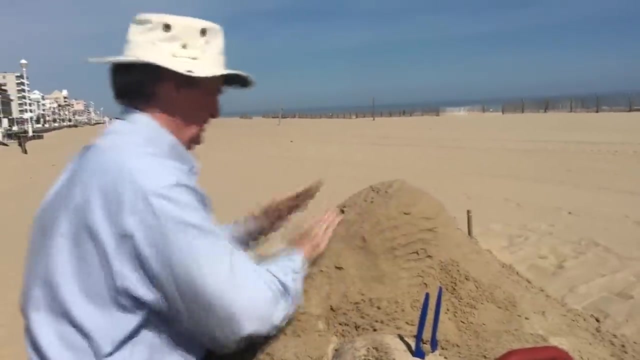 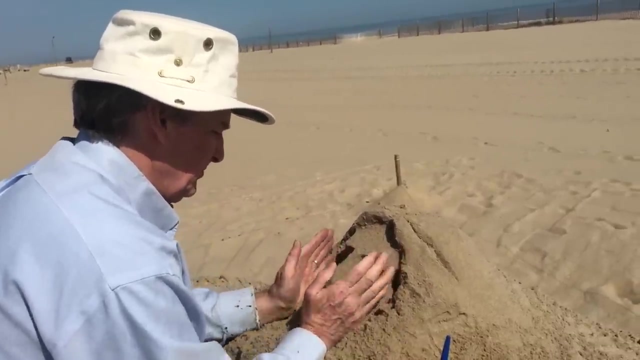 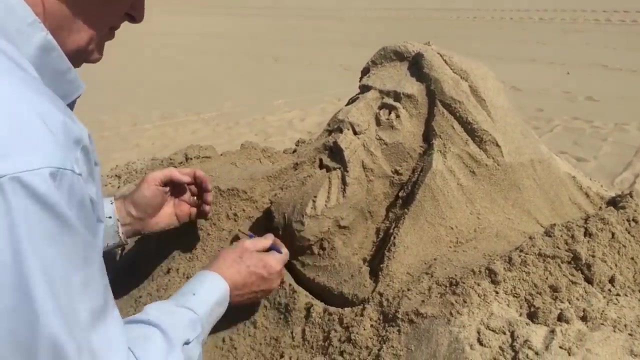 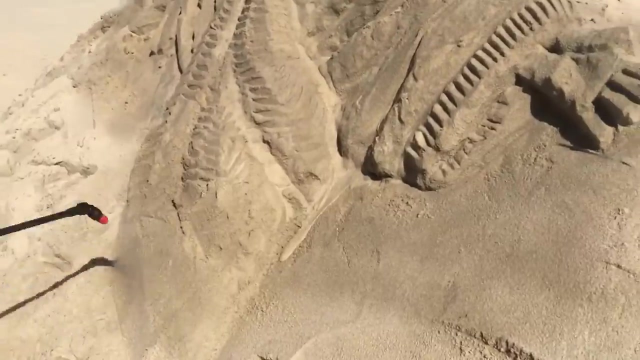 sand sculptor, Randy Hodman works throughout the day to create a biblical masterpiece- Number 6.. This great god is alive again at a beach in Ocean City, Maryland. Professional sand sculptor, Randy Hodman works throughout the day to create a biblical masterpiece. 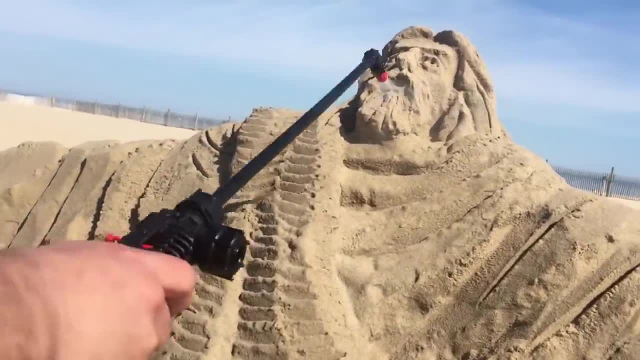 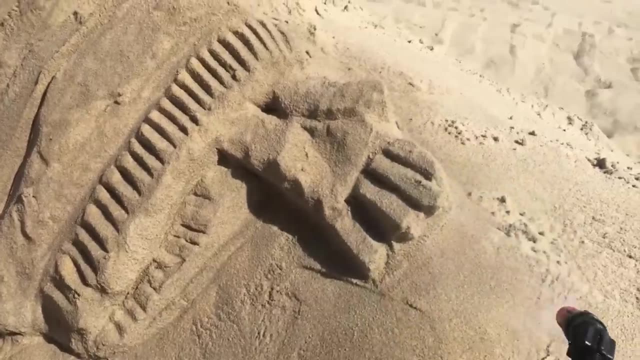 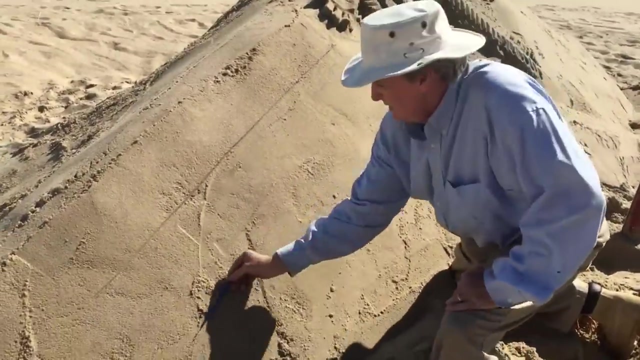 This great god is alive again at a beach in Ocean City, Maryland. Professional sand sculptor Randy Hodman works throughout the day to create a biblical masterpiece, Number 7.. This great god is alive again at a beach in Ocean City, Maryland. Professional. 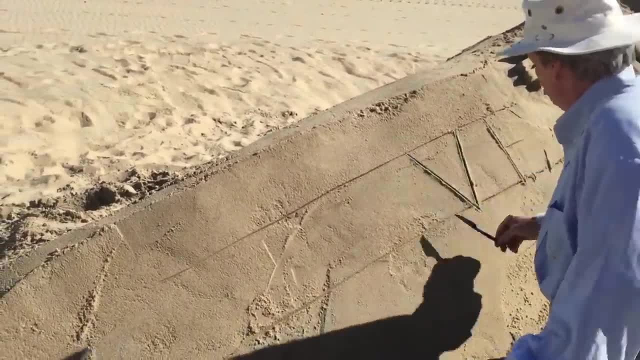 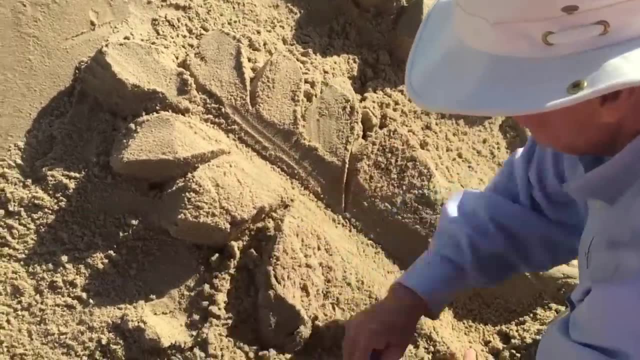 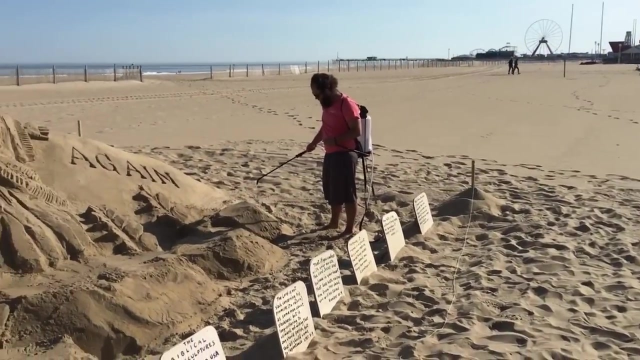 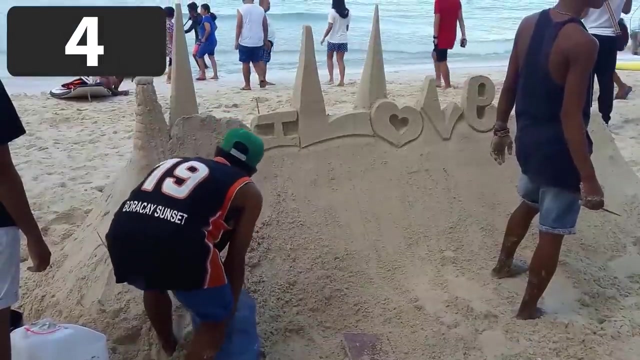 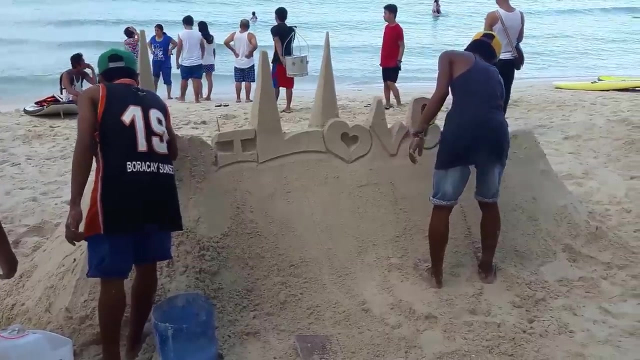 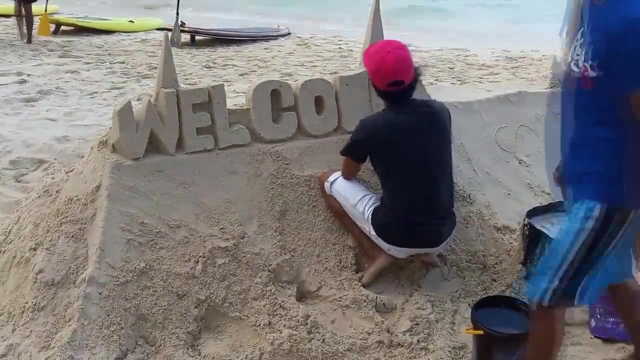 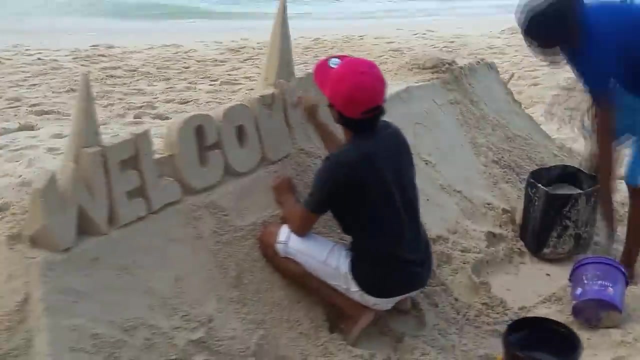 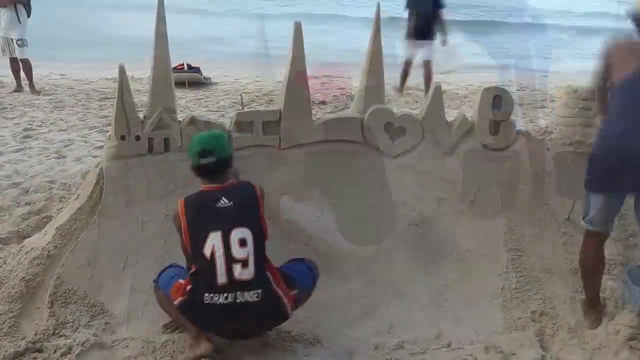 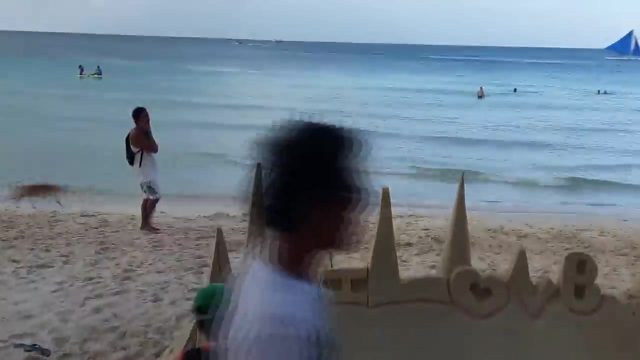 Number 4. Boracay is an island in the Philippines with a proud and patriotic native people. To show their love for their island, they create a beautiful sandcastle. They mostly use their bare hands, but also use a carving file. Boracay is the name for the northernmost island in the Philippines. 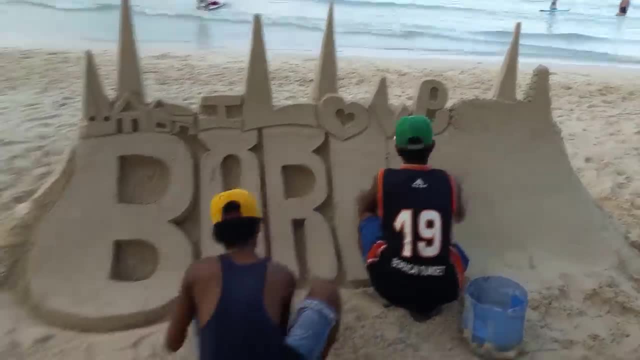 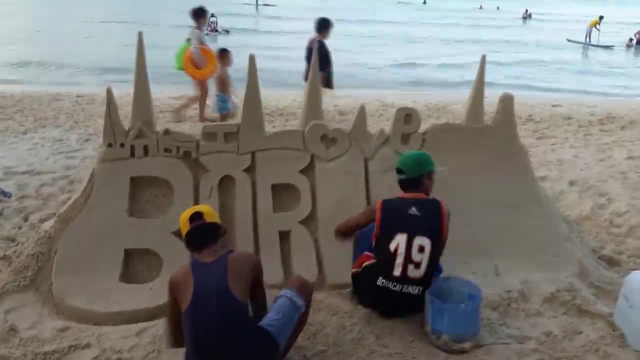 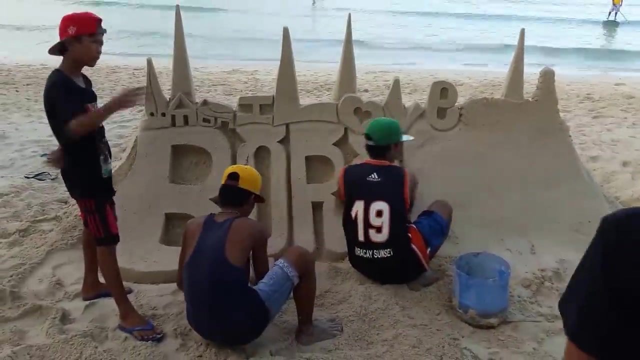 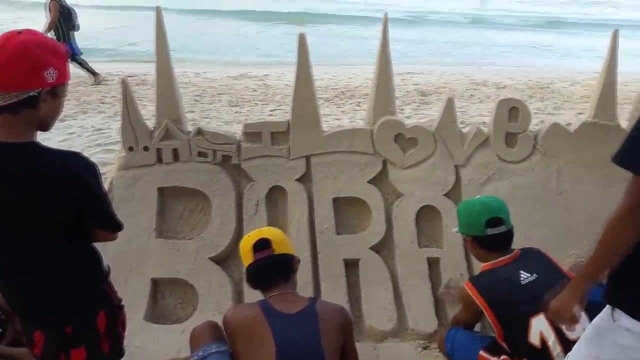 Boracay is the northernmost island in the Mediterranean Sea. Boracay is a population of not only British River Islands, It is also a históric territory, not only Mediterranean but also Indian. Boracay is the ne' Boracay is the place to visit when you travel around the world. 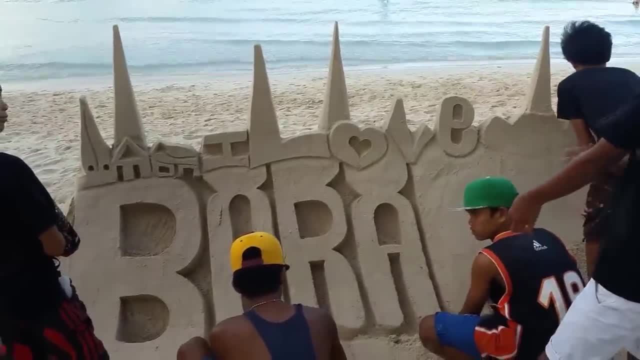 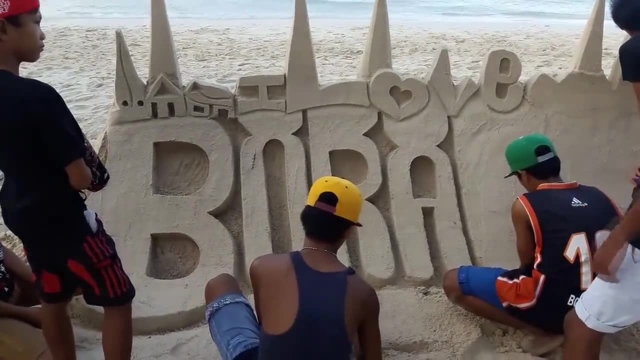 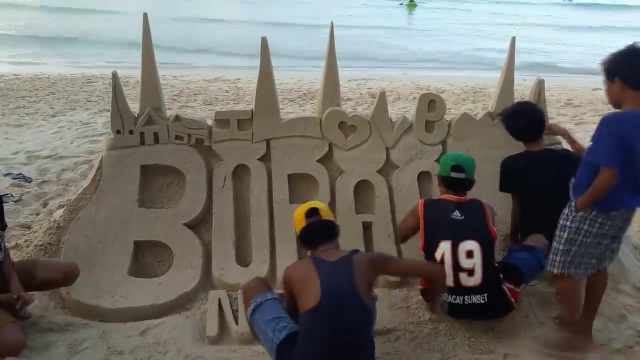 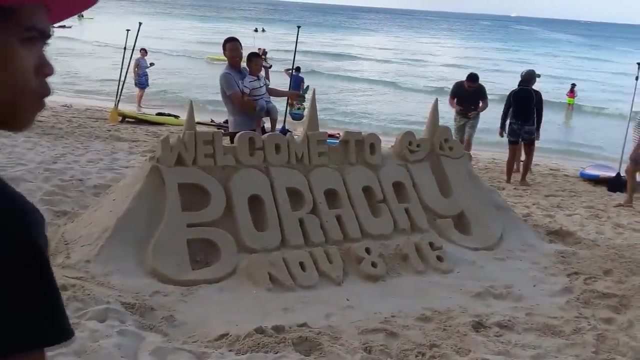 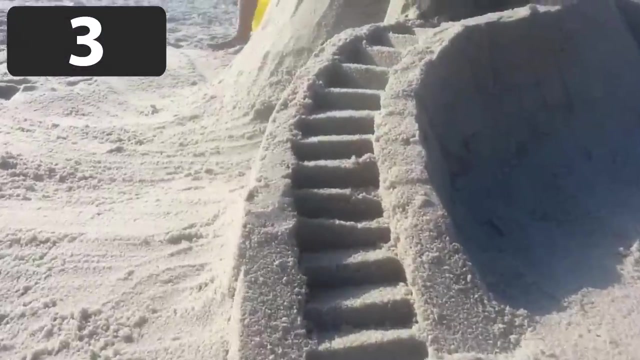 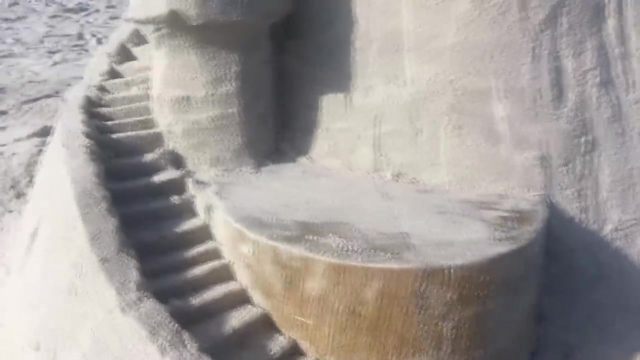 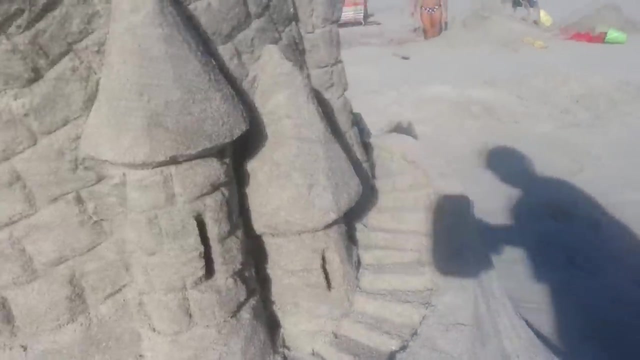 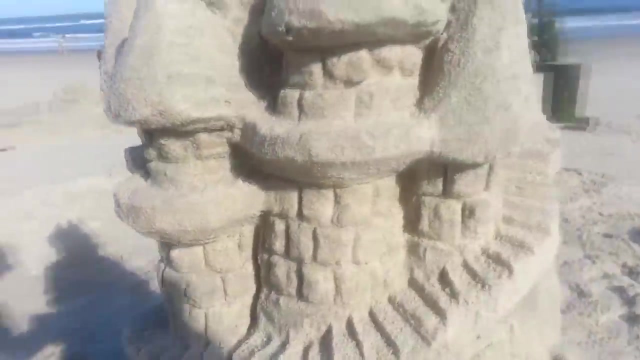 so. so number three: it took around seven hours for these beach goers to recreate the disney castle in the sand. they used a small sand shovel to do most of the work, but also used a special sand tool to do the brick work and the fine details. a straw was also used to blow away unwanted sand. 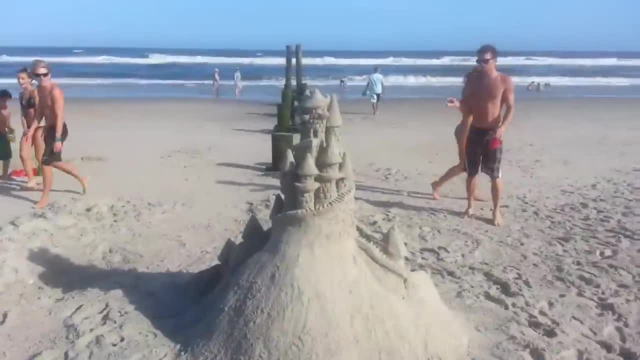 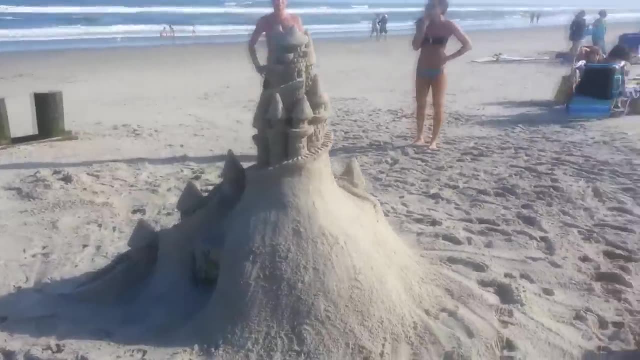 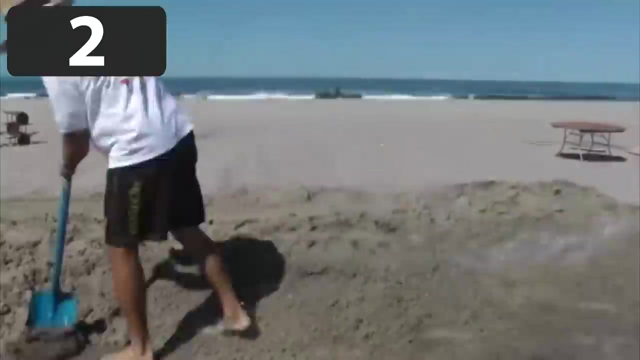 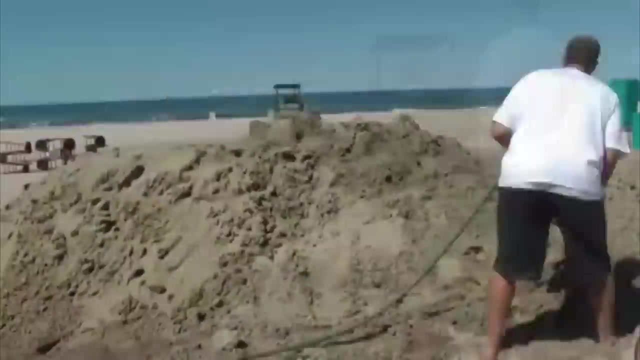 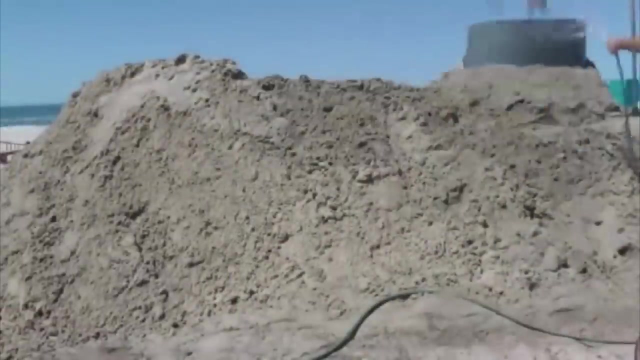 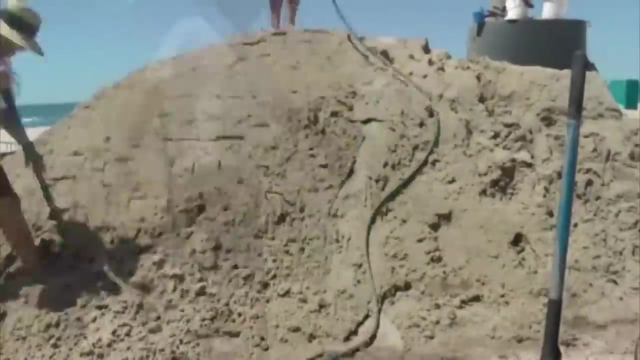 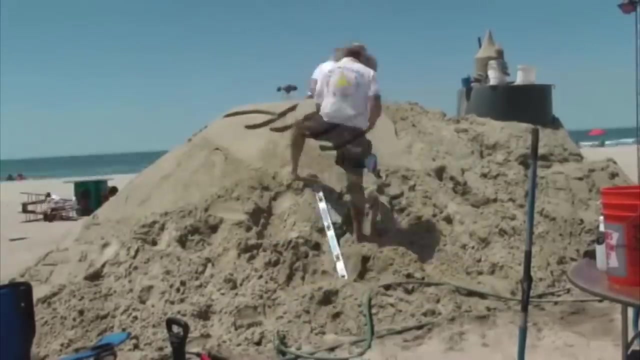 so i'm making like two or three videos per castle. number two: archa sand is a company that designs professional sand castles for corporate events and parties. this time lapse footage shows the creation process of a massive sand castle they built in california. they even used a bulldozer to help build. that's some serious sand making. 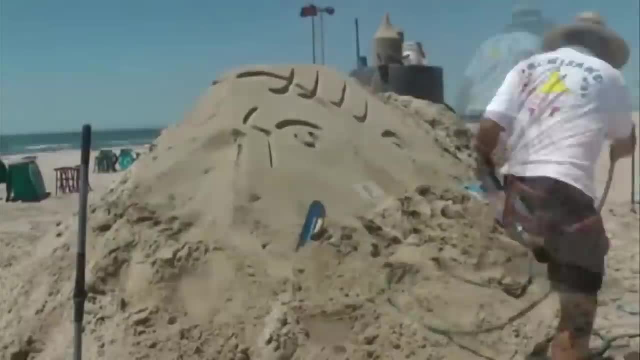 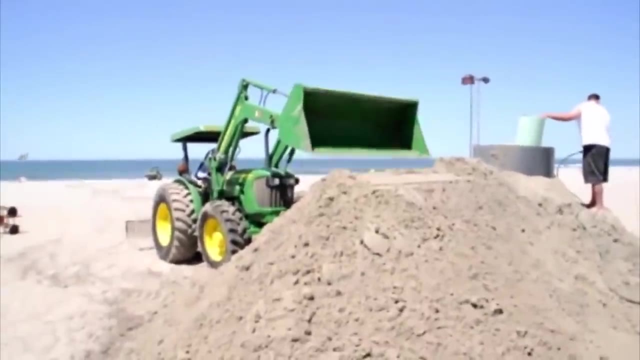 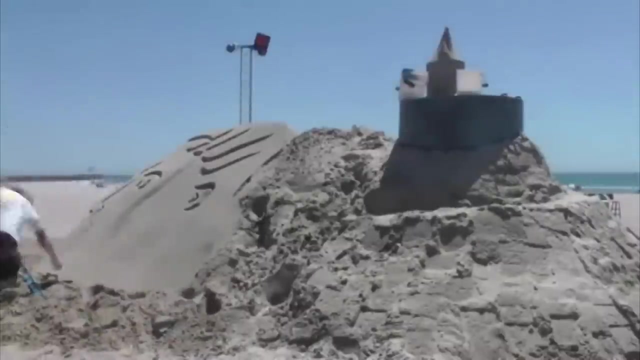 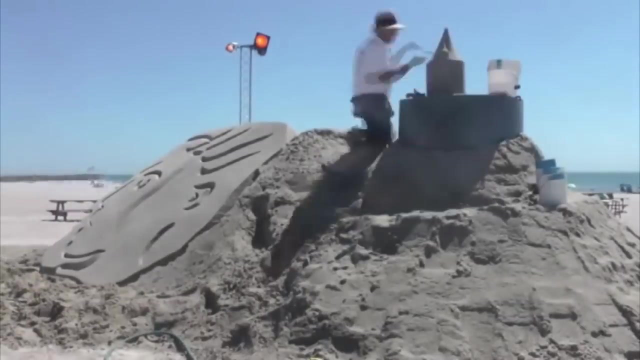 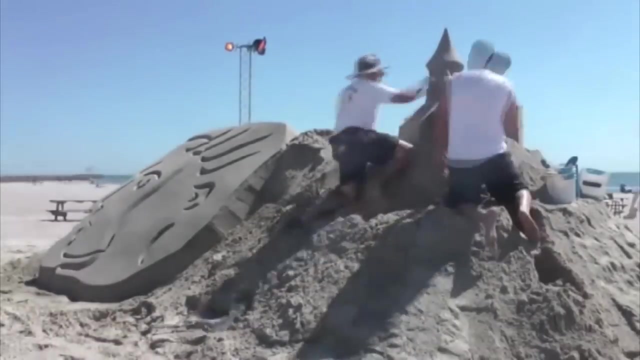 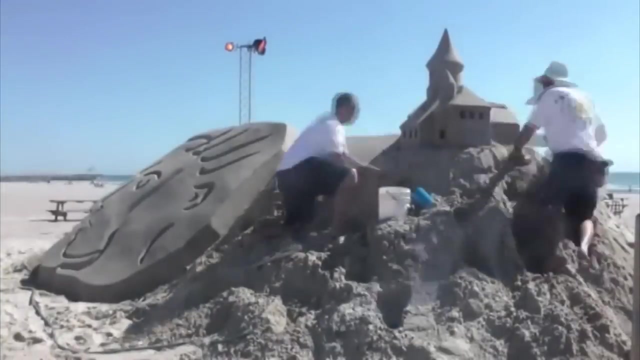 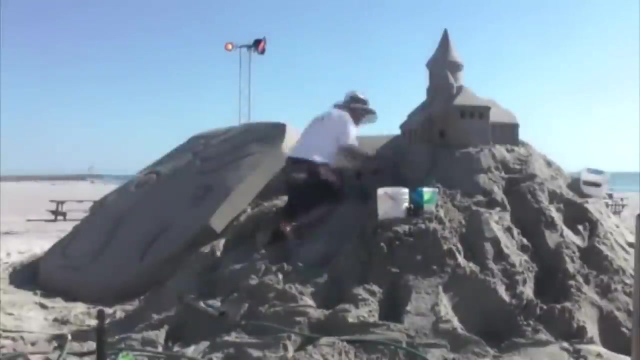 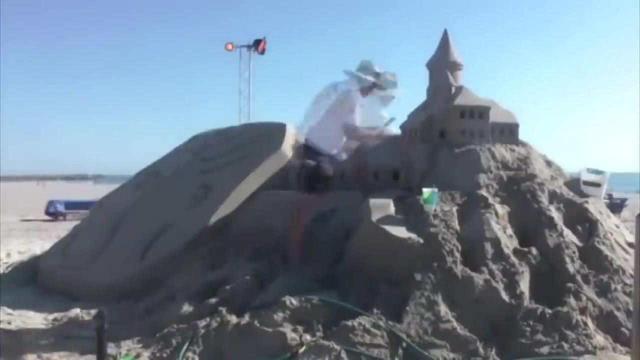 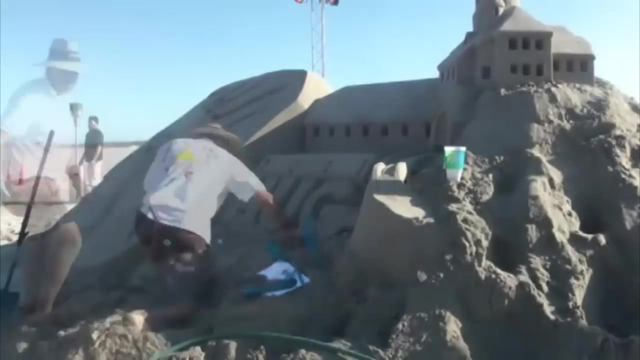 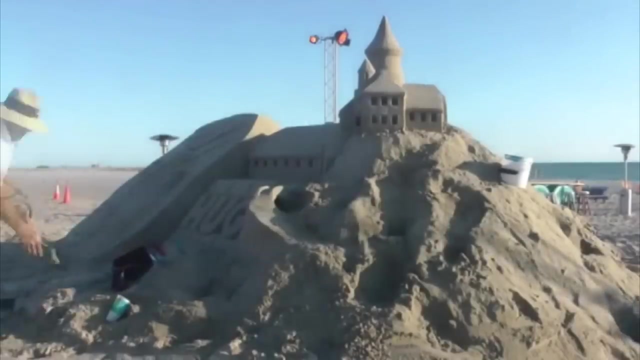 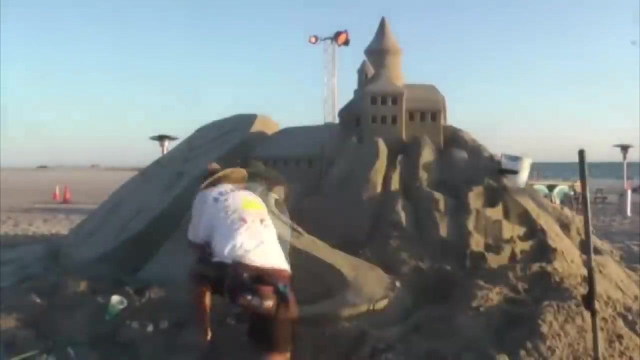 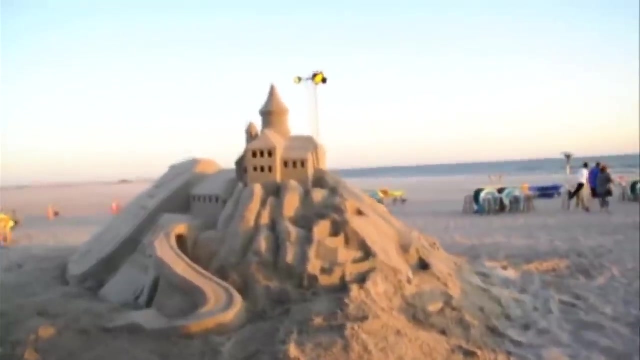 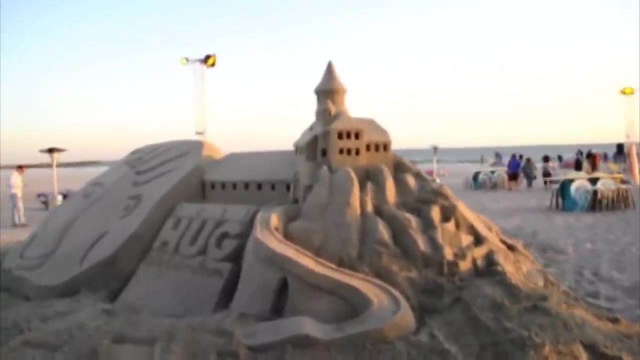 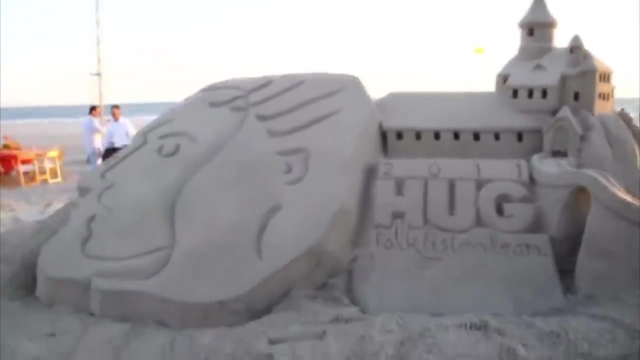 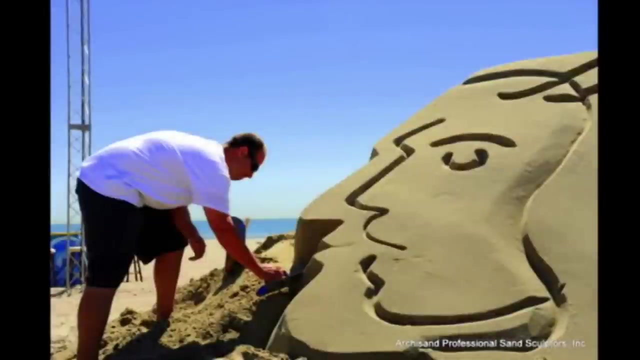 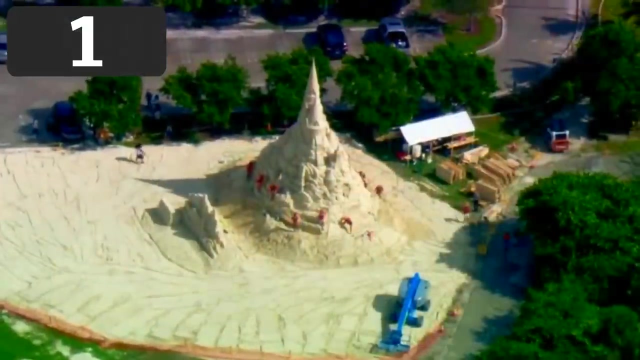 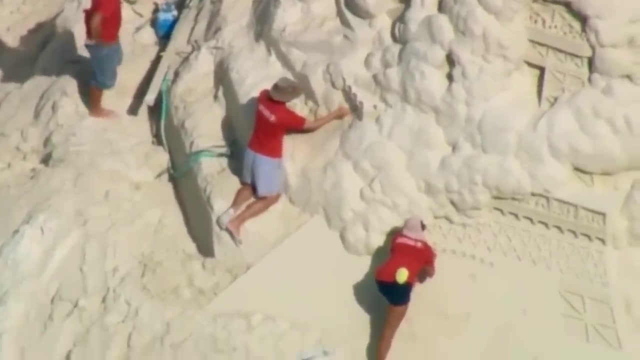 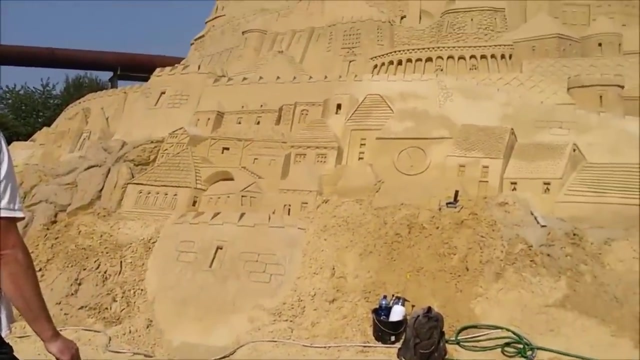 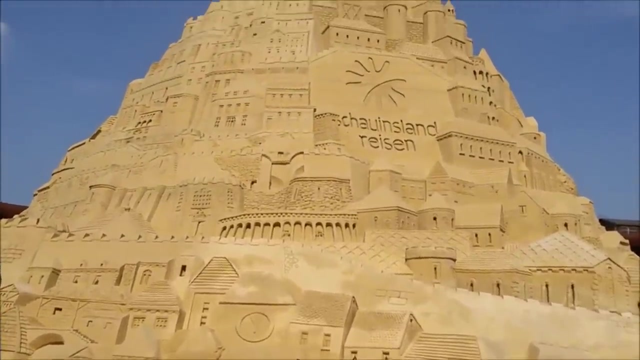 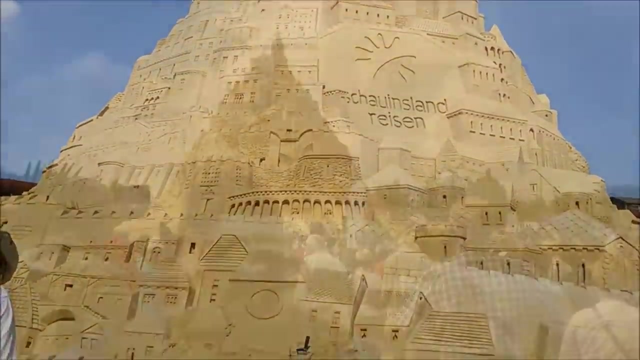 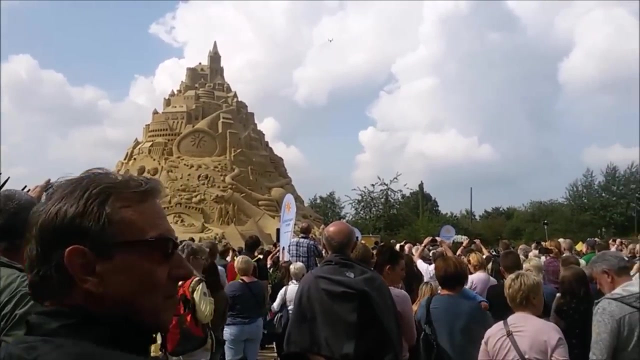 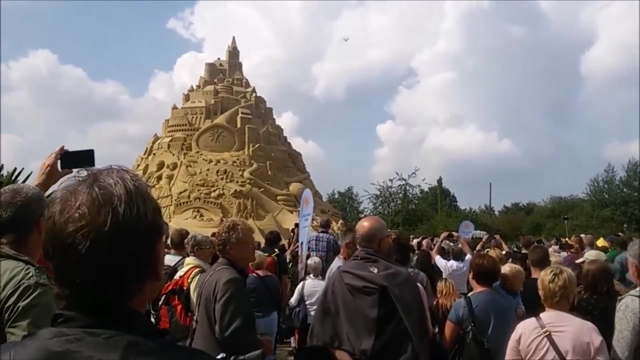 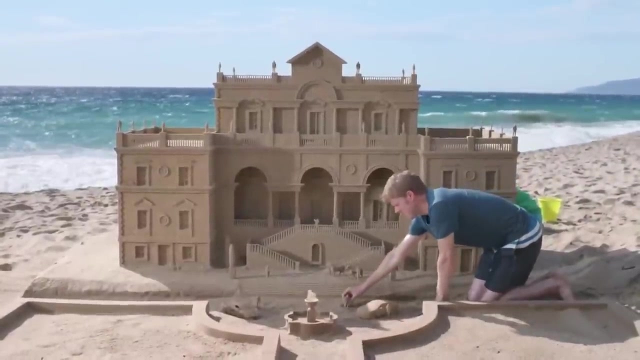 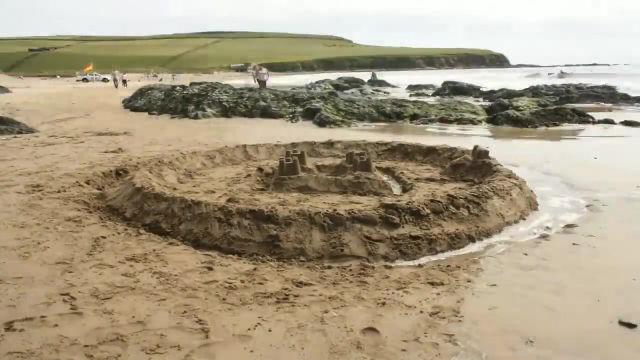 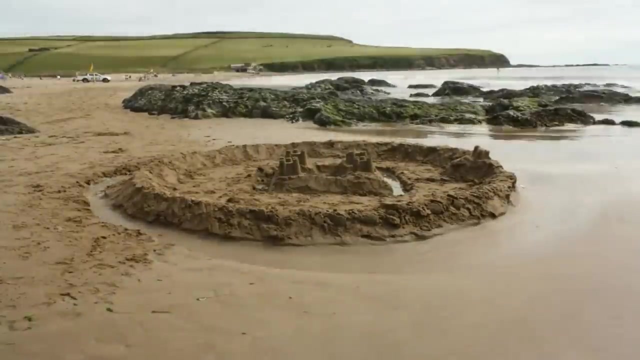 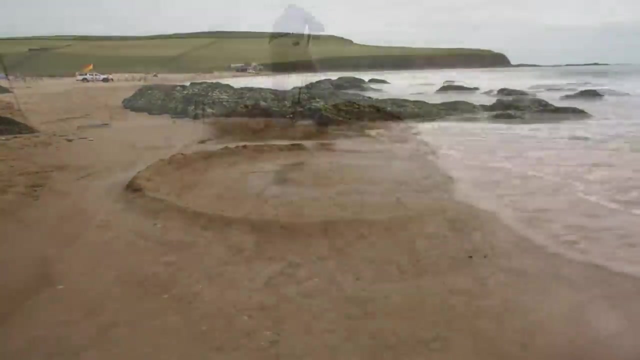 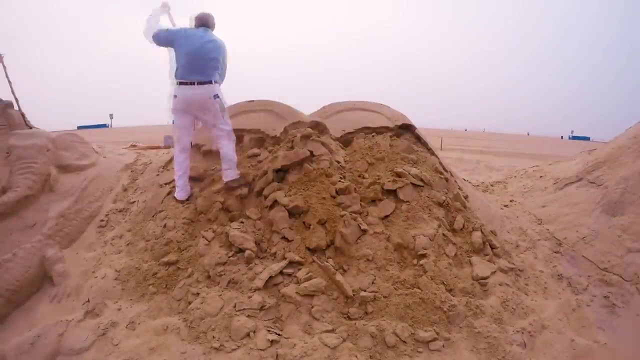 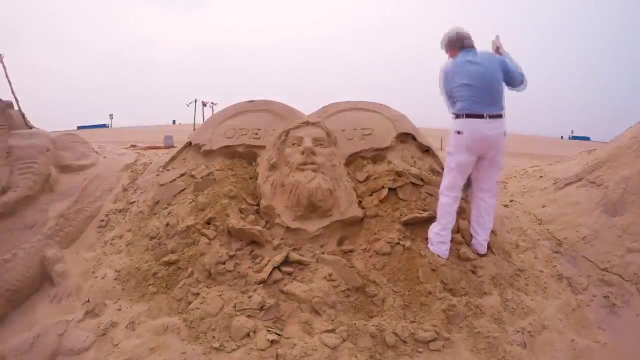 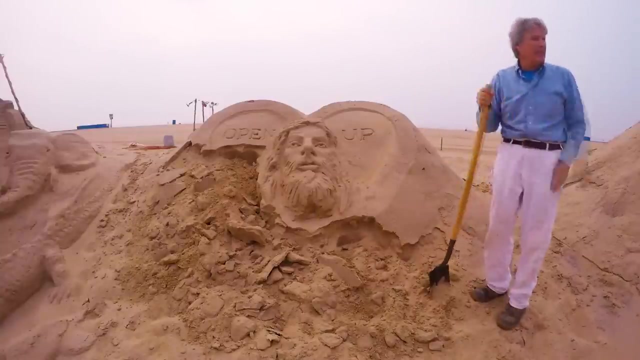 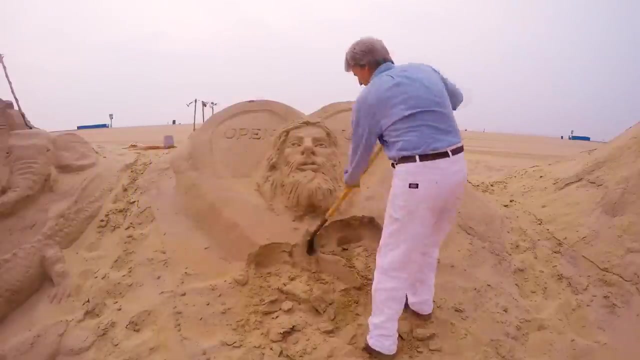 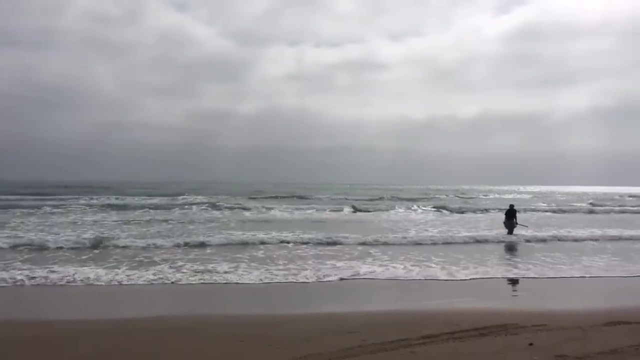 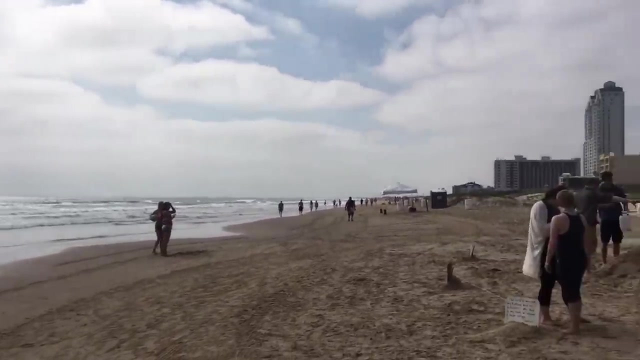 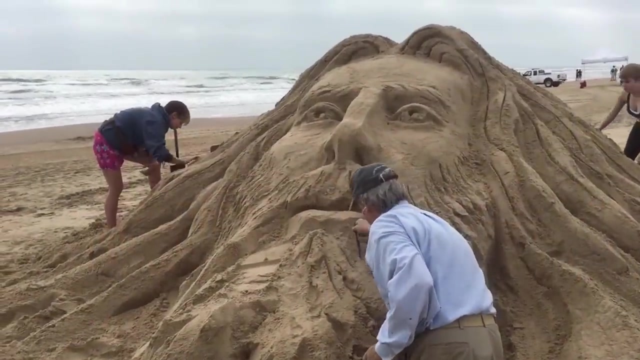 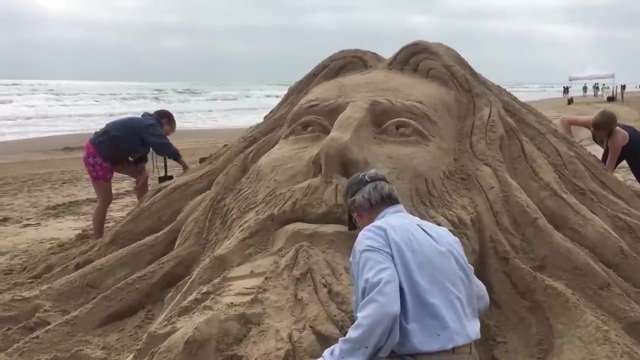 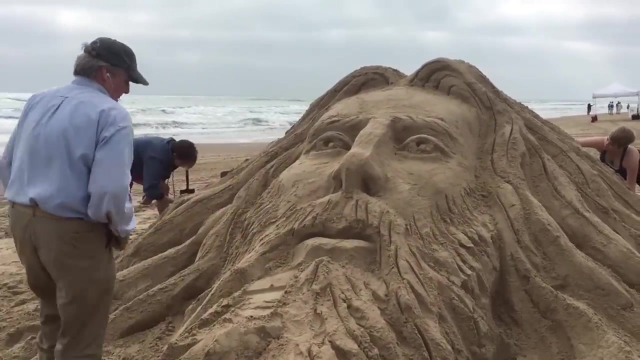 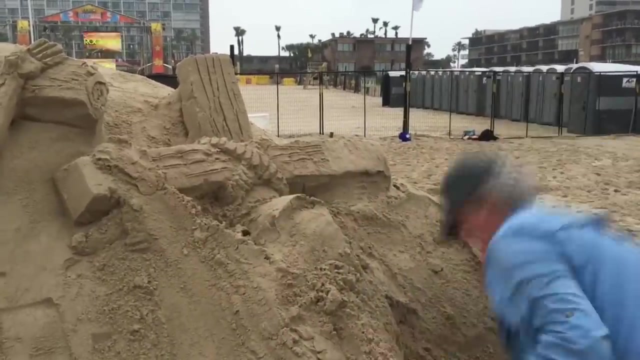 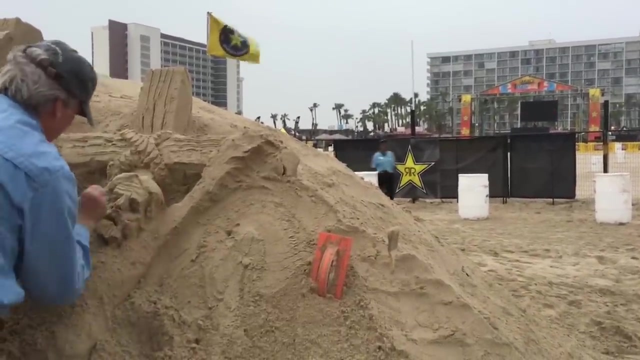 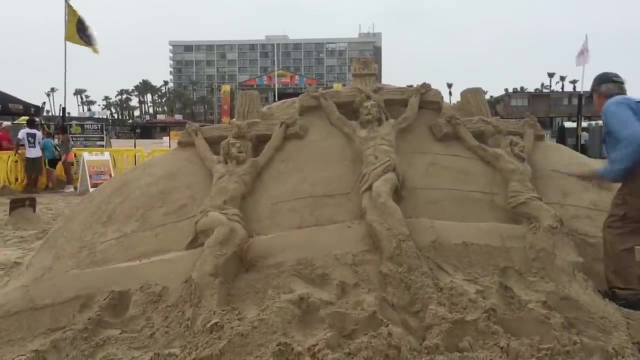 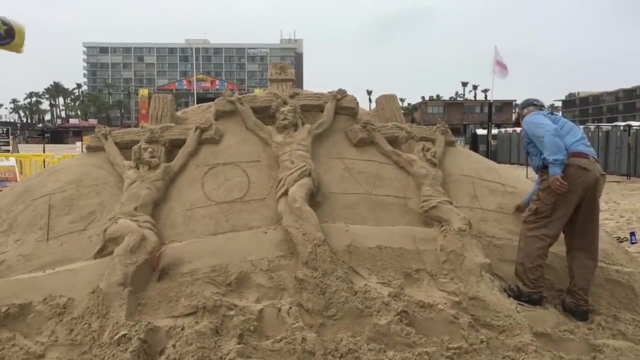 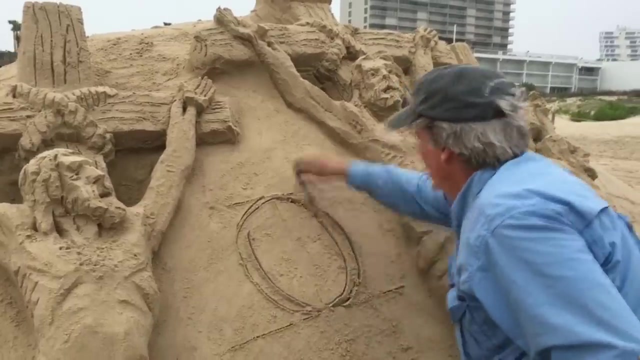